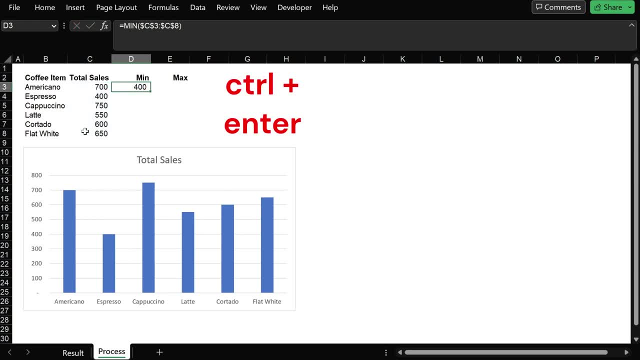 when we drag the formula down And then we're going to press control enter, I'm going to stay on that same cell. come to the corner, drag the formula down. Now we're going to do the same for max, So I'm going to input max. 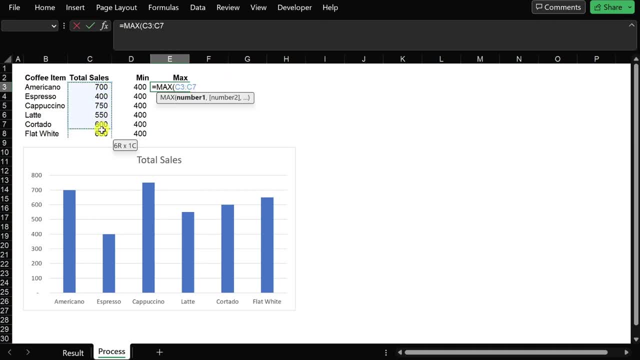 press tab so it auto completes the formula. Again, I'm going to select the information. press F4 to lock the cell so they don't change when we drag the formula down. Control enter to stay on that same cell and then drag it down. So now you've got the minimum and maximum value for. 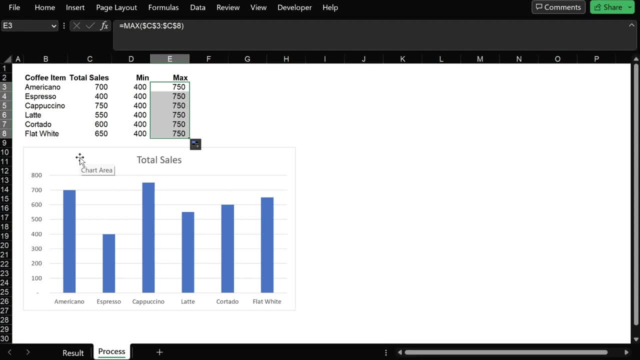 the information provided. So when I come down to the chart, I'm going to click on it and it's going to show you what information forms part of it. And we want to include the minimum and maximum values. So you can see at the corner, when we bring the cursor down, it changes to a diagonal arrow. 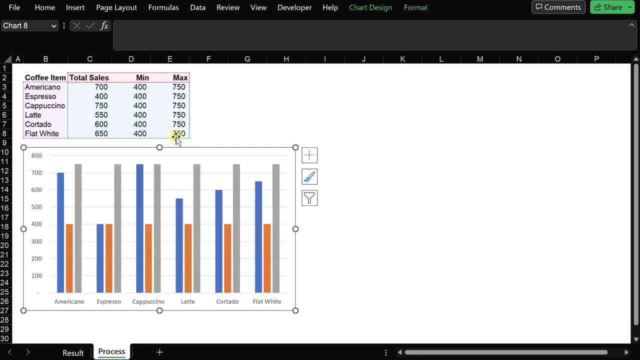 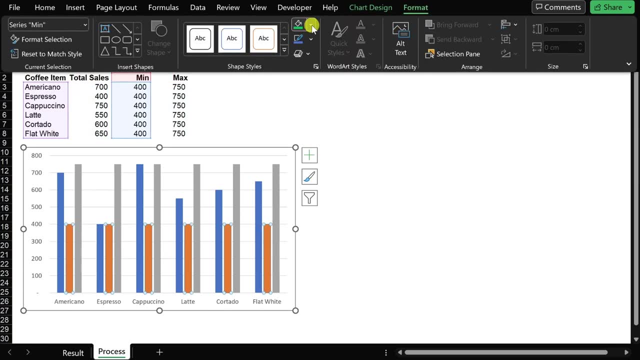 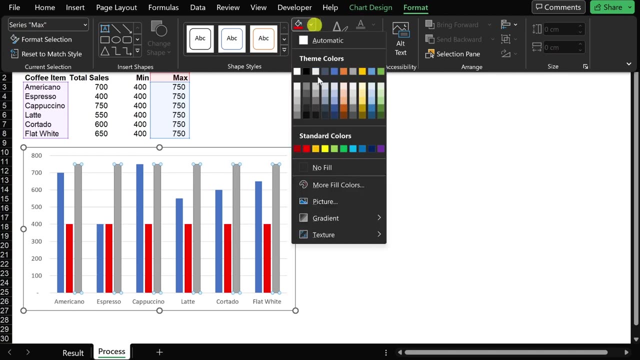 I'm going to drag it so it includes minimum and maximum, and now it's one part of our chart. So while we're busy, let's just change the colors: Minimum, we want to change into a red, and maximum we're going to change into a nice bright green. The problem we have now is we've got 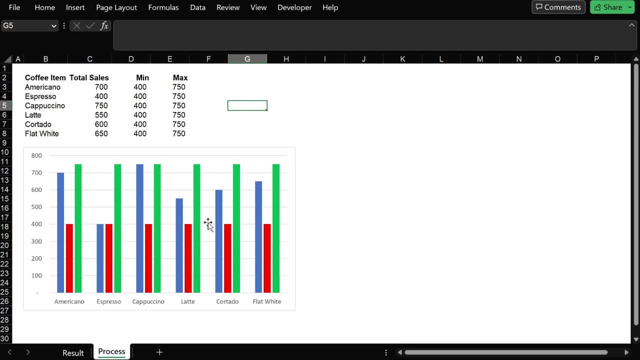 the minimum and maximum value at every single chart item, and we only want this for the actual minimum and maximum value. So to do this, we're going to come back here to the formula. I'm going to cut this portion out just so it's easier to follow along. 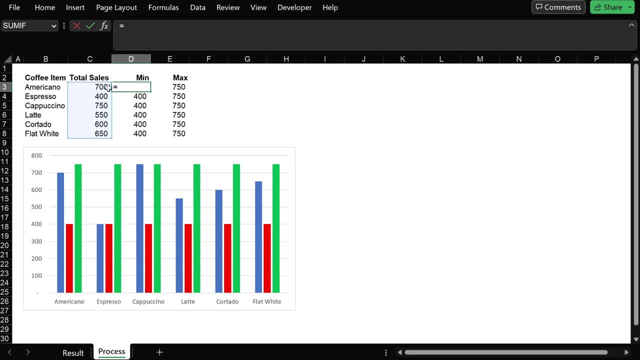 To do this, we're going to use an if formula that states that if this is the minimum value, please return it in this cell, otherwise return nothing. So I'm going to say, if tap to auto complete, this value equals, and then I'm going to paste that value that I just cut out. 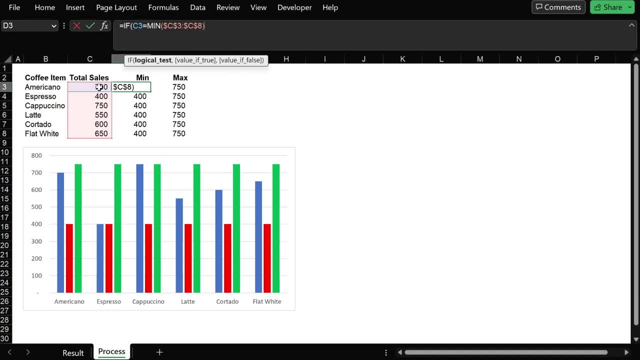 So if that value is the minimum of all the values in the range, then give me that minimum value, otherwise give me nothing. So blanks, two quotation marks, not a zero. Zero is recognized by Excel as a value, So I'm going to paste that value in the cell and then I'm going to paste it. 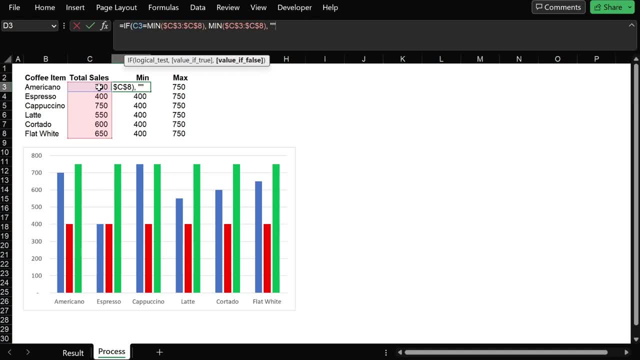 This is a value and will then be included into the chart and then close the bracket Again. control, enter to stay on that same cell and you'll see now it's blank because Americanas are not the minimum value. So when I take this formula and I drag it down,